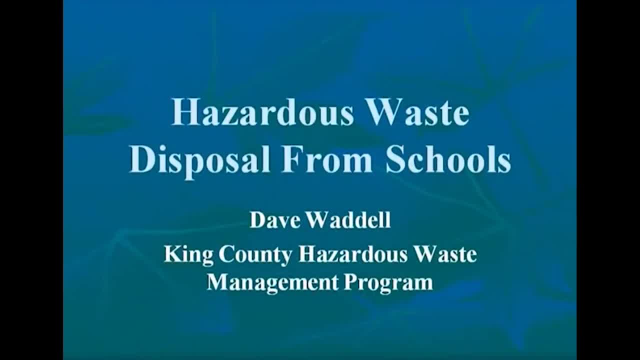 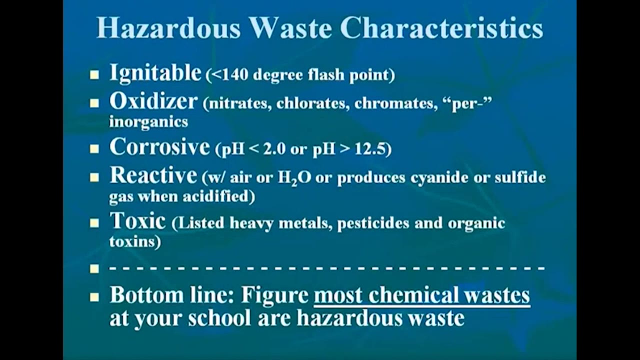 started on hazardous waste management from schools And I realize this is probably one of the driest topics and I'll try to spice it up a little bit so it's not just reciting regulations to you. Washington state has extremely rigorous hazardous waste laws. Only three states in the union have. 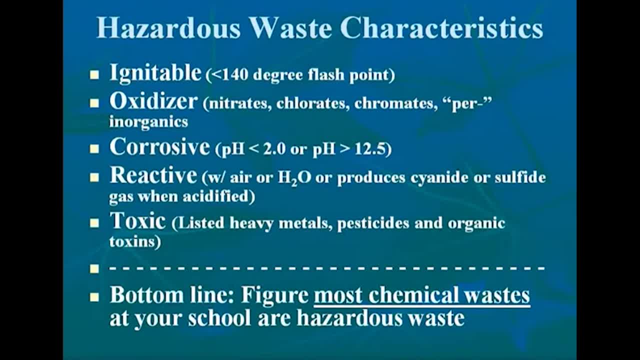 hazardous waste regulations that are as stringent as ours are California, Minnesota and Washington. I've posted on this first slide that there's ignitable and oxidizers and corrosive bases and corrosive acids and reactive compounds and toxic compounds, And all of these are the characteristics. 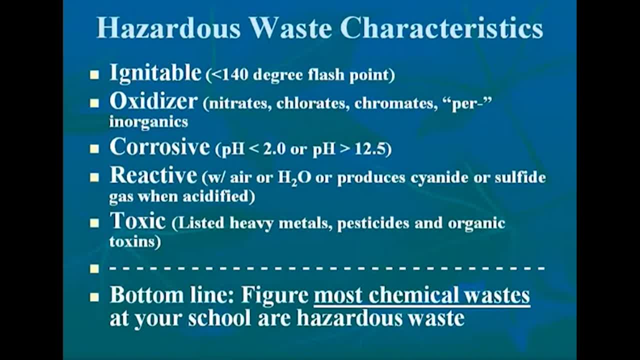 of hazardous waste. So things that burn at room temperature very readily, things that cause other things to burn, things that will corrode your skin if you touch them, whether they're basic like Drano or like an acid. things that if you spit on it, breathe on it, it bursts into flames, or if 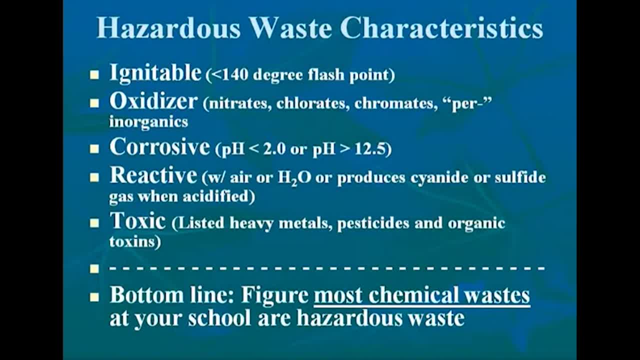 you twist the cap, it can blow up, And things that if you swallow it, you touch it or you inhale it can cause you to become either very sick or actually die. These are the kinds of characteristics we're worried about in hazardous waste regulations. 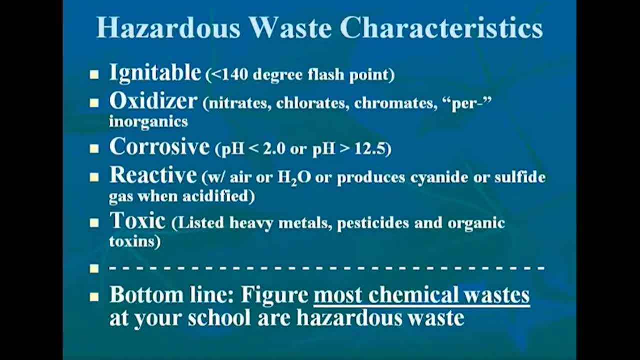 But the bottom line that you should know in Washington state is virtually everything in your school that is a chemical if you try to dispose of it is probably going to designate as a hazardous waste. It's kind of like mushrooms in the wild. The odds are not good that you just pick up some random mushroom and it's going to be edible. 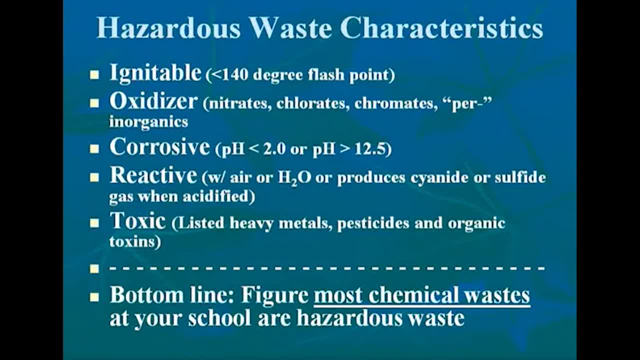 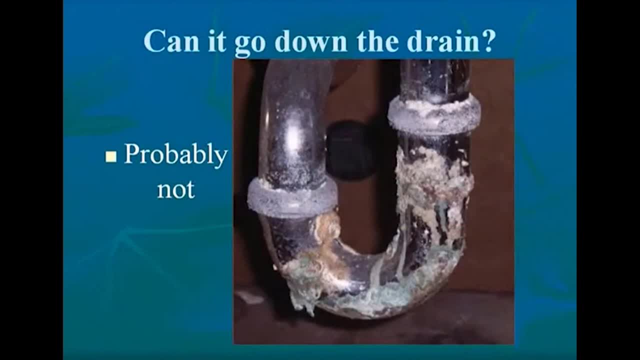 The odds are even lower than that. The odds are even less good that you would take any chemical you've got and throw it in the dumpster, and that would be a legal disposal option. So, given that, let's talk a little bit about what you can do with this stuff. 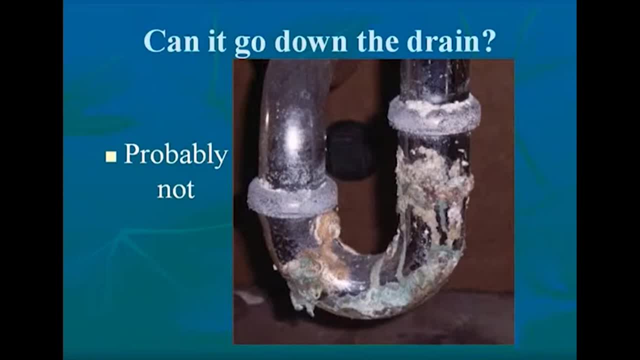 So can you pour your chemicals down the drain when you're done with them? Probably not. Again, most of them are going to be designated as hazardous waste, and you can't pour hazardous waste down the drain unless you've got a permit from your local sewer authority. 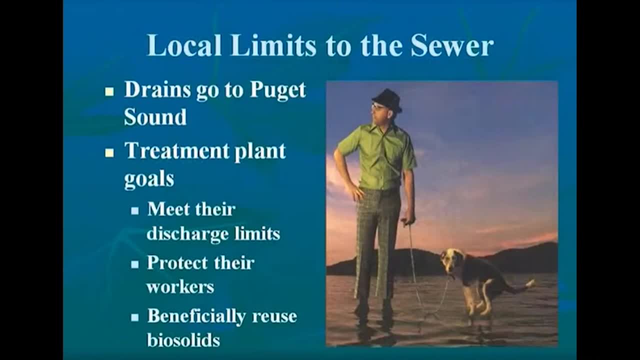 They don't issue those permits very often and you've got to pay a lot of money for it, And the reason they don't do this is the drains go to Puget Sound, which is the largest sewer in the state. The drains go to Puget Sound or they go to local lakes or streams and the treatment plants are also under restrictions from the federal EPA on what they can allow to go out into the receiving waters. 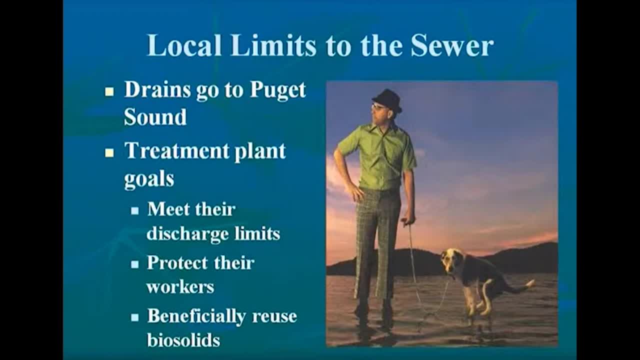 So they don't want anything coming into the treatment plant that may cause them to be regulated as being an illegal, hazardous waste disposer. They also want to protect their workers, and anything that does get trapped in there is going to go into the biosolids that may get applied to beer fields in eastern Washington. 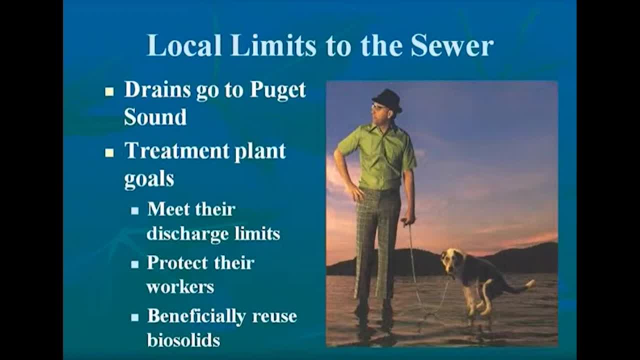 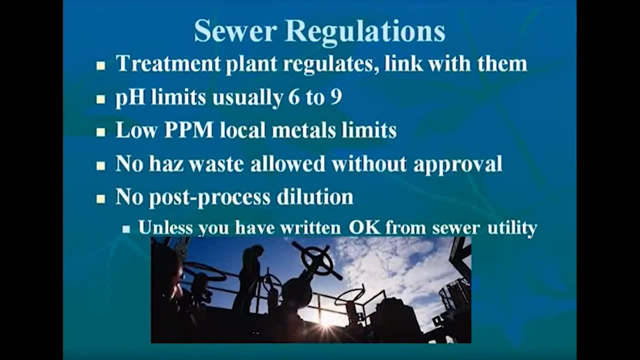 And I like really clean beer. So no dumping. You're toxic Heavy metals into the drain. So what are sewer regulations like? Well, the treatment plant regulates it. So if you want to know, call your local treatment plant. You can figure that out by just asking your accounting department who they're sending their payments to as far as paying a sewer bill, 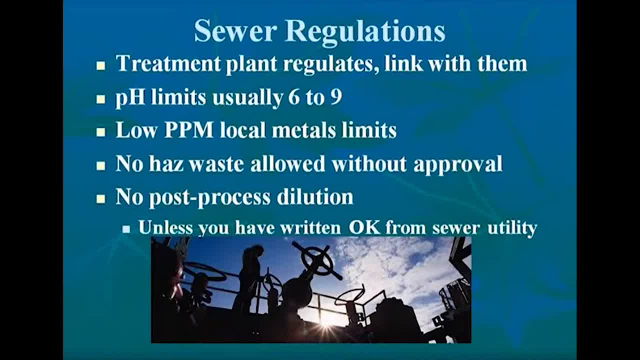 The pH limits are usually between 6 and 9.. Some of them expand a little bit, but unless you've got something that's between 6 and 9, it's either too corrosive basic, too corrosive acidic to go down the drain. 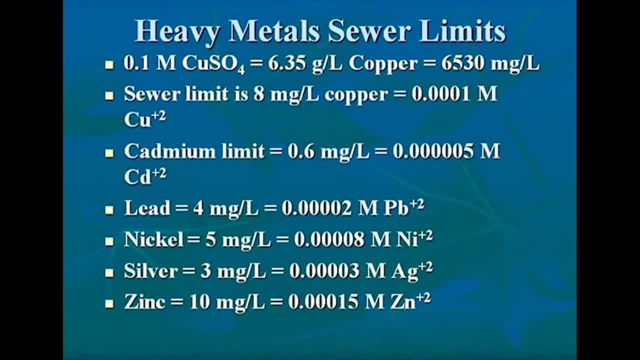 Heavy metals are the ones People tend to put down the drain And the limits for what can go down are at the low part per million level. Incredibly dilute before it's OK And nothing that would designate as hazardous waste without approval. 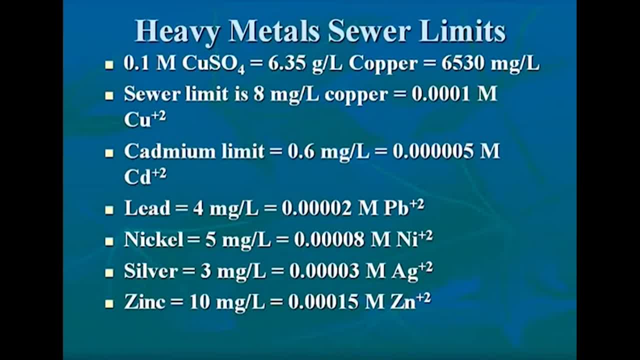 The other thing to understand is just because you can add a whole lot of water to something to make it more and more dilute doesn't mean it's OK. That is considered evading the intent of the regulations and is illegal at the federal, state and local level. 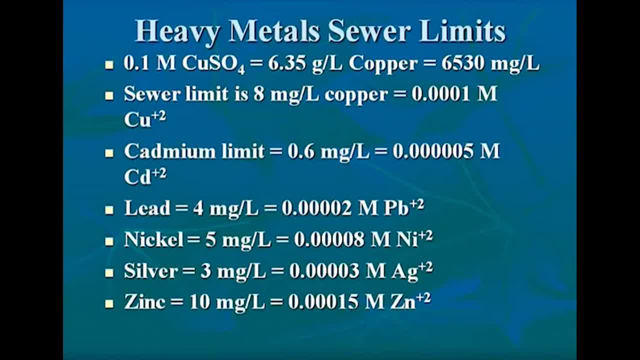 So unless the sewer utility has specifically written you something in writing that says it is okay for you to dilute this particular material and put it down the drain, You can't do it. So when I'm talking, dilute part per million concentrations of heavy metals, what does that look like? Well, most science teachers are familiar with. 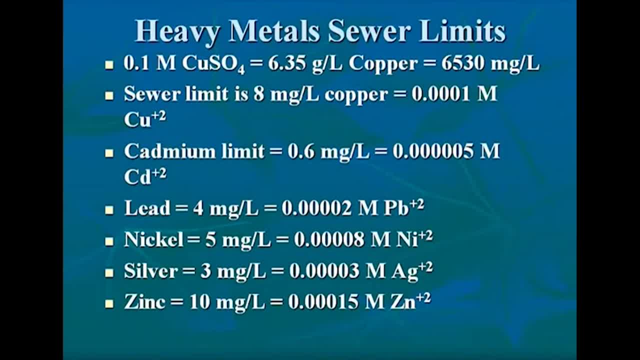 things in molarity, And the most dilute molar solutions we see people work with are typically 0.1 molar, So copper sulfate, one of the most commonly used chemicals in the science lab. you're working with a 0.1 molar copper sulfate solution. That's got to be okay to go down the 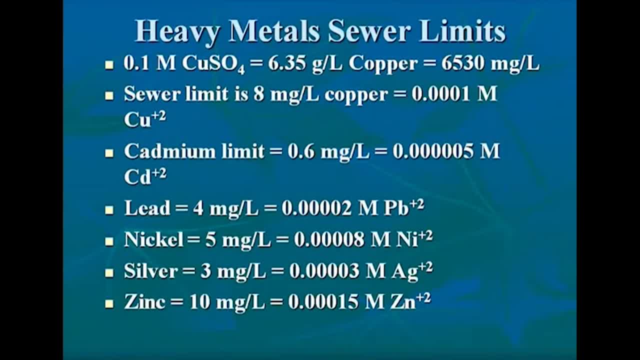 drain right? Well, let's work out the calculation. And when you do, you realize that 0.1 molar copper sulfate is 6,530 milligrams per liter, which is equivalent to part per million of copper. Most sewer agencies have a sewer limit of 8 milligrams per liter for copper, So 6530 versus. 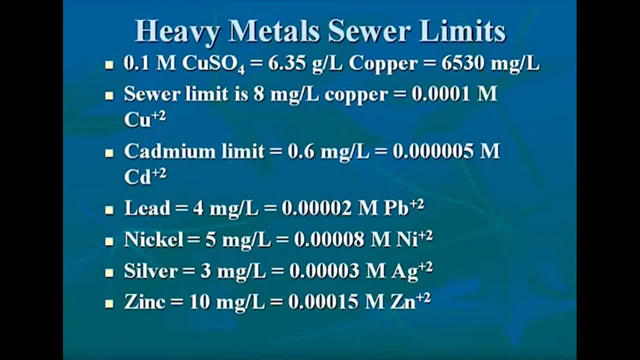 8, you're 800 times the allowable concentration of copper that can go down the drain. Now you could always try to dilute that pint of 0.1 molar copper sulfate you've got with 800 gallons of water. if they say it's okay, Of course, then you're going to have to find. 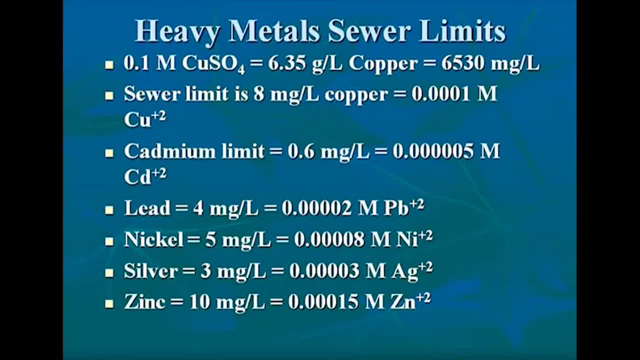 someplace where you can hold 800 gallons of dilute copper sulfate before you discharge. You can't just pour it down the drain and leave the sink running. You have to treat it by diluting it first. I'm thinking you don't have an 800-gallon tank in your science classroom to do this. 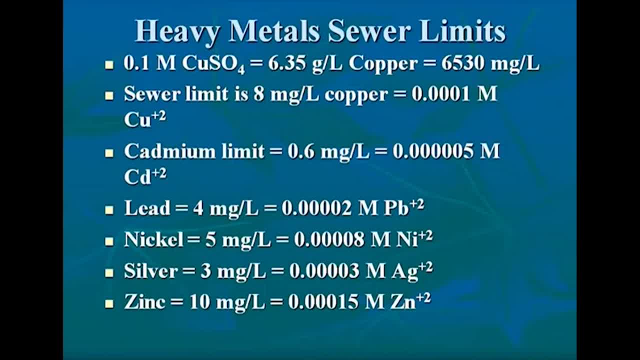 Cadmium level is even crazier. You'd have to have a 0.0000005 molar cadmium solution in order to have it go down the drain. When I show this to science teachers, I keep getting the response: well, at 0.0001 molar, it's not going to do. 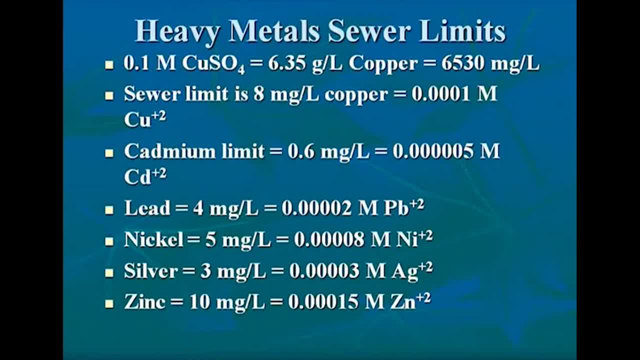 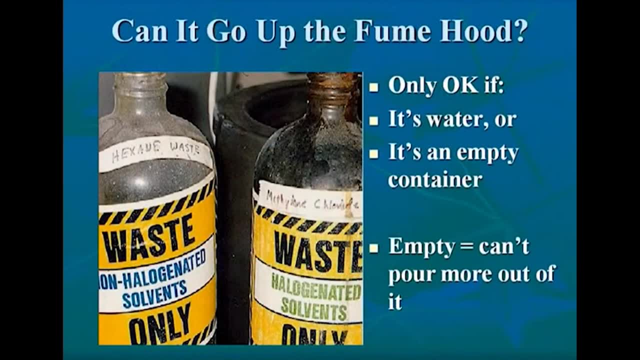 anything. Exactly That's why it's safe at that concentration. So if I can't pour it down the drain, maybe I can evaporate it. Well, it's okay to evaporate your waste if it's the water that you're evaporating out of it. Or if it's the water that you're evaporating out of it, you can evaporate. 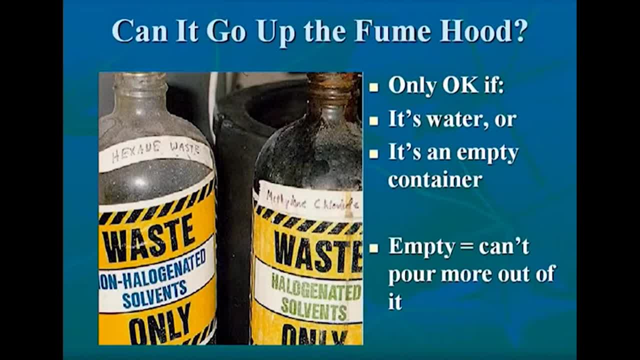 it. It's a completely empty container where you've poured everything you can out of it and you're just trying to dry it out a little bit. Aside from that, no way. So you can't evaporate your flammable solvents, even though they're volatile. That's illegal disposal under the 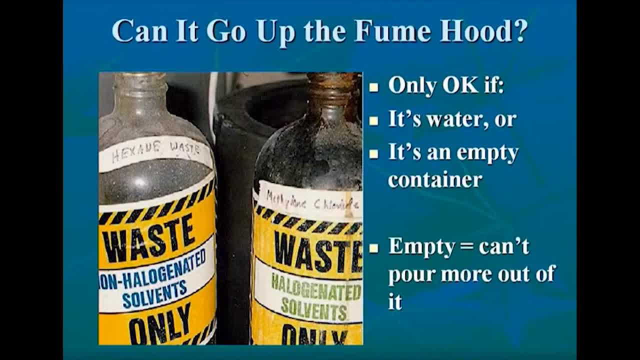 Clean Air Act. So if I can't pour it down the drain and I can't throw it in the trash and I can't evaporate it up in the air, what can I do with it? Well, there are some options that. 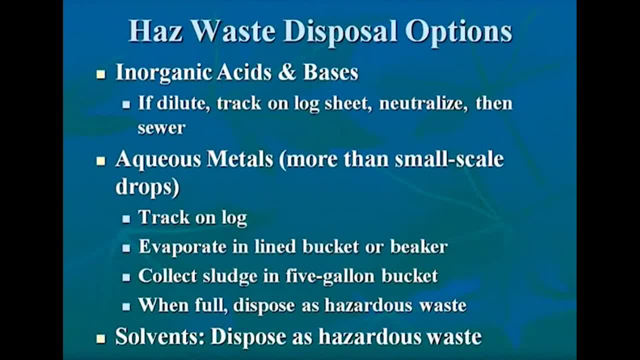 you have prior to disposal that you can do. The first one is, if you've got acids and bases, that you can dilute them very carefully, track it on a log sheet, neutralize them and then pour them down the drain if they don't have any heavy metals or other types of contaminants in it. 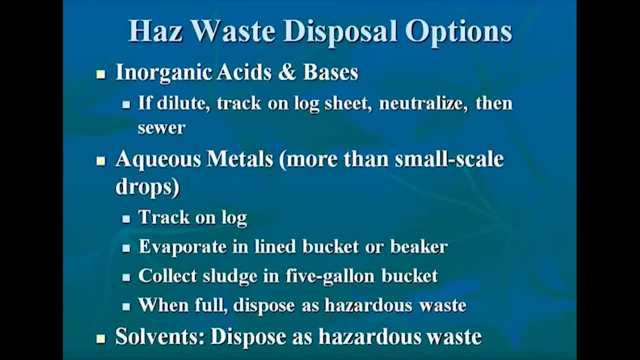 For the aqueous metal solutions more than just a drop on a sheet of paper that you can wipe up with a paper towel, these can be evaporated. My recommendation is that you track this on a log so if somebody like myself who's a hazardous waste inspector comes in and says 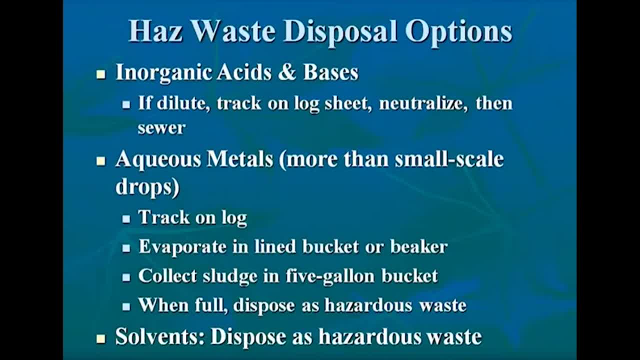 so what do you do with your metal solutions? You say, oh, we properly dispose of them. Prove it. If you've got a log sheet saying what you're doing and you have records and receipts from the disposal, then I'm going to be convinced. 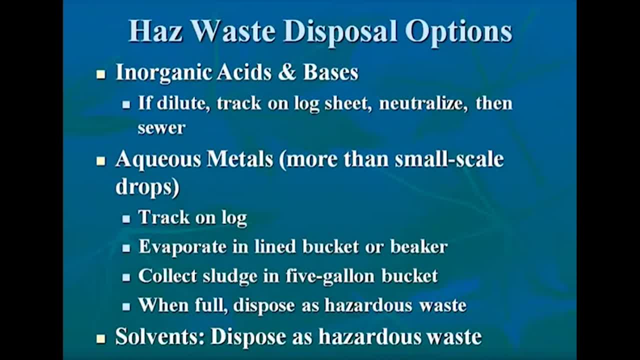 Other than that, I'm thinking you're either pouring it down the drain or you're dumping it in the backyard. So keeping a log sheet shows me, as an inspector, that you're doing the right thing. And schools are regulated exactly the same as any other business. There's no exemption for. 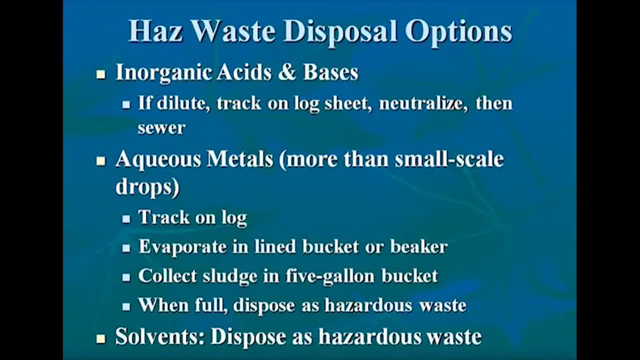 schools under the hazardous waste regulations. So you can be fined and penalized and all of that stuff, just like any other company. So if you've got a log sheet saying what you're doing, you're dumping it. So what I recommend for the aqueous metals, which is the most common: 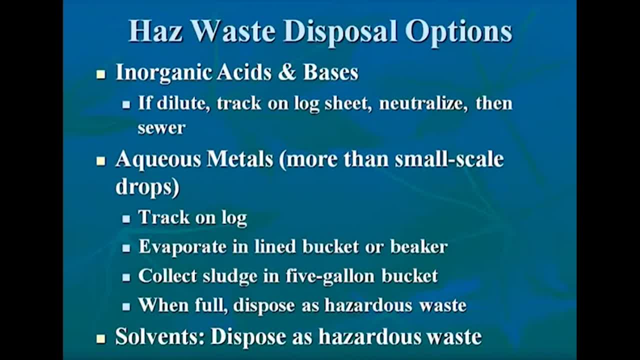 waste stream you probably have from your science labs at least, is to get a Ziploc-type baggie, a good-sized one, line a beaker with it. pour any of these liquid metal solutions you've got into that bag and let them evaporate. 99.5% of the solution you've got is water, So you're. 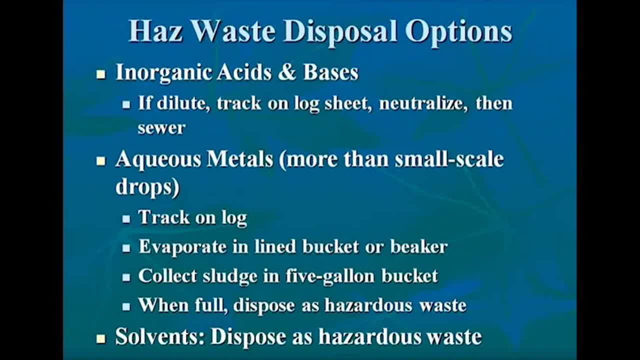 reducing the volume by 99%, which is going to save you a lot of money. Once you've filled the Ziploc bag with sludge, zip it closed, lift it out of the beaker, put it into a plain five-gallon paint. 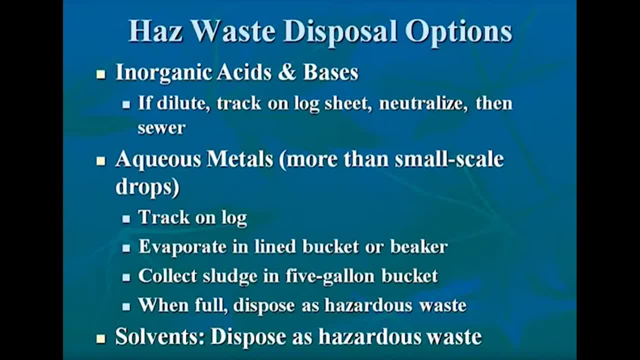 bucket, snap the lid on and write the words hazardous waste- heavy metal salts on the top. When that bucket's full, then you can dispose of that as hazardous waste. For a typical science lab it'll take you 40 years to fill that bucket, Costs you about $250 to dispose of it, So $4 a. 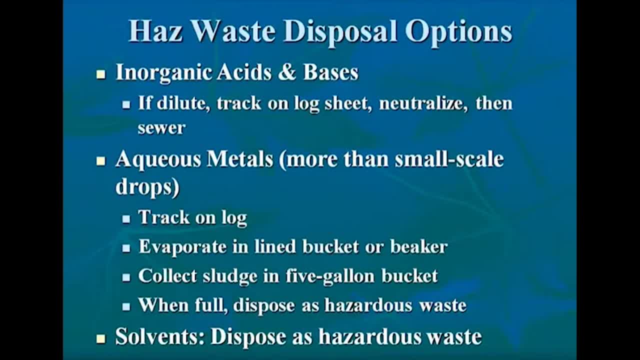 year for your hazardous waste budget. It's pretty cheap, So I don't want to hear any whining out there about how tough this is and we don't have a budget. Trust me, you can afford this one. Solvents are different, though. If you've got flammable solvents, those you need to collect. 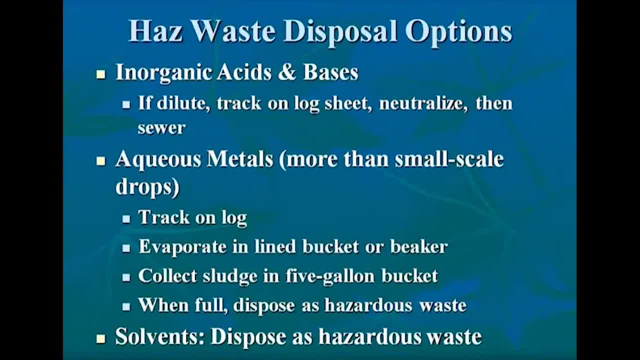 typically back in the original bottle. So keep an empty solvent bottle around to use as a waste bottle. Write the words hazardous, waste flammable solvents on the outside and then collect your waste solvent in there. If you can avoid having waste solvent, that's great. It'll save you some. 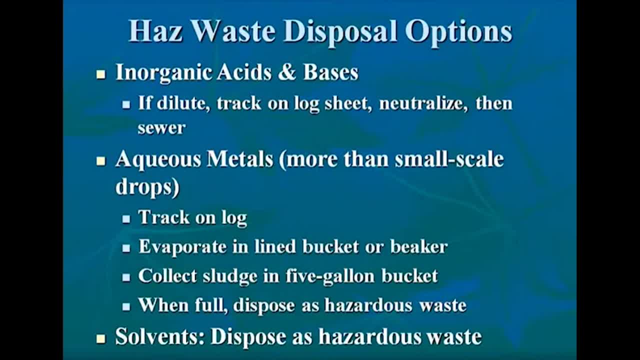 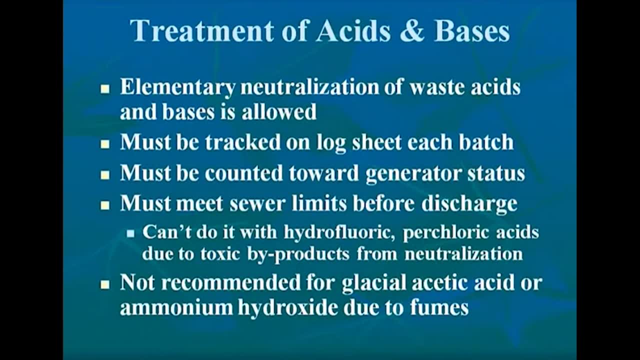 money. Solvents will go off to be burned as fuel, So it's not a real expense. It's not a real expense, It's a very expensive disposal option again. As far as acids and bases, again they can be neutralized. You need to track it on a log sheet, One of the ways you could do this, though. 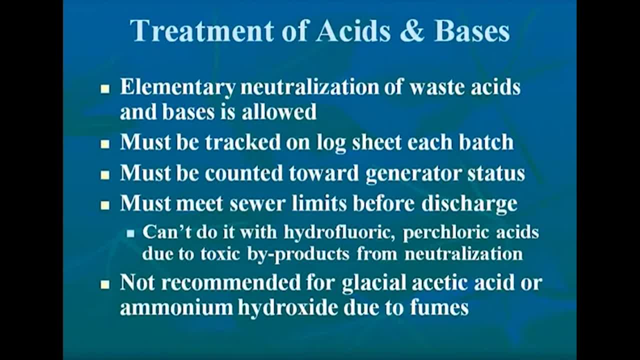 is you could actually do it in class, because if you're a chemistry teacher, you're probably teaching acid-base neutralization reactions. Why not use your waste acid for this or your waste base for it, rather than something new? Now, it's teaching, It's not disposal. You don't. 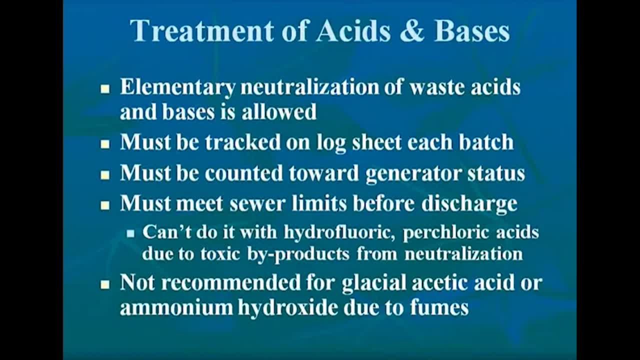 have to track it, You don't have to count it. Once you're done with that lecture or the experiment, then you determine whether the material is hazardous waste If it's been neutralized, between six and nine go down the drain. 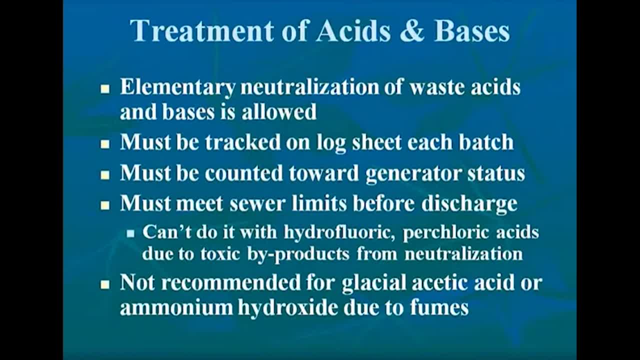 Now there are a few acids that you can't use it on. Hydrofluoric acid, which we talked about in the high hazard chemical section, is way too dangerous to be doing acid-based neutralization. Percloric acid, which is a very toxic compound and highly reactive also, is another one that 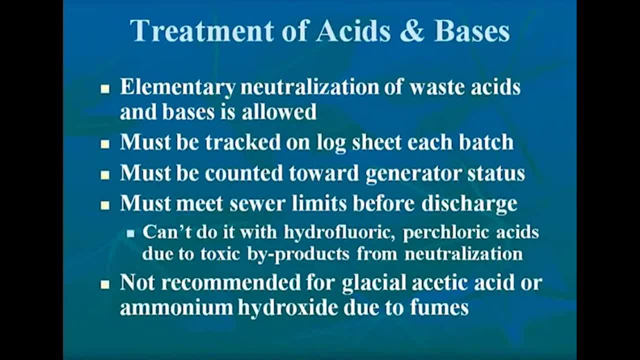 you probably don't have, And if you do, you can't do this type of neutralization because the reaction can get a little too hot. Glacial acetic acid and ammonia hydroxide are two other corrosives that we don't recommend being neutralized, just because they generate a lot of very stinky fumes and you really 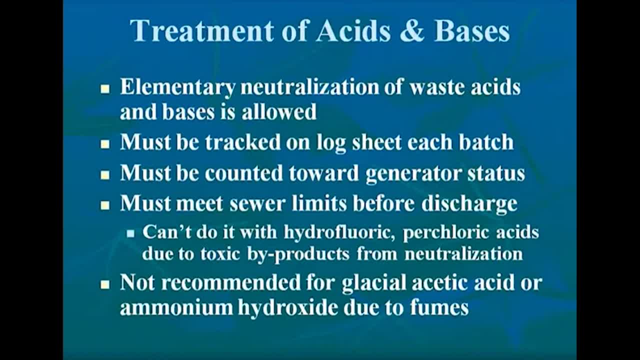 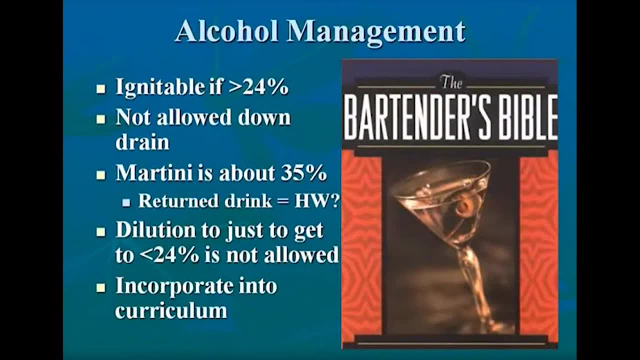 wouldn't want to have the ammonia vapors flying all through your lab. Now I always get asked about alcohols. It's like, okay, alcohols can't go down the drain. What's that about? And the point is well made. 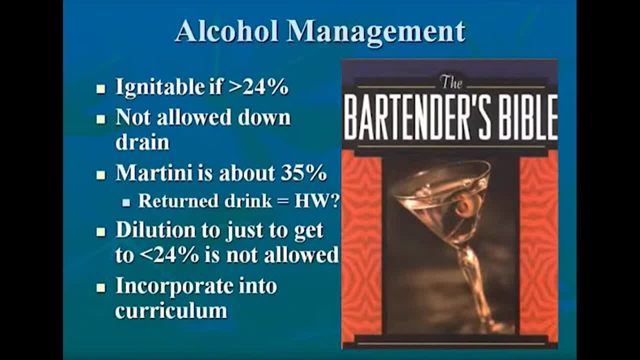 If you go to a typical bar, the example I always use is: I'm at the bar, I order a scotch on the menu. The bartender rocks. They deliver the scotch. I look in. One of the ice cubes has a fly suspended in it. 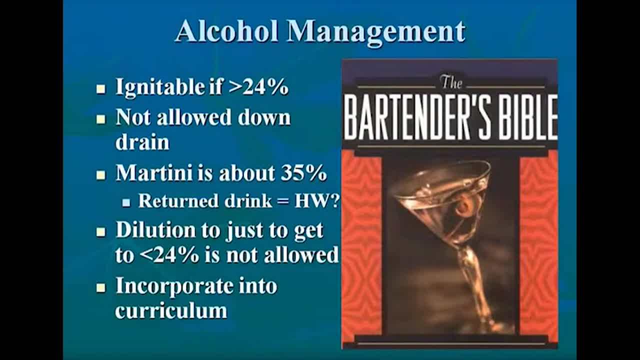 I give the drink back to the bartender. What does the bartender do with it? Well, alcohols are considered ignitable hazardous waste. if they're over 24% in concentration They're flammable liquids. They're federally regulated by the EPA as a flammable hazardous waste. 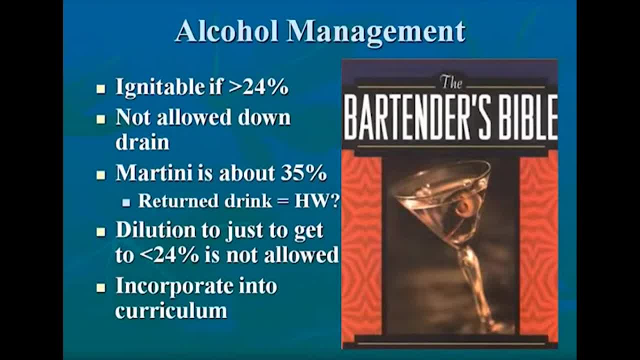 So a bar is a business. So he takes back the martini or the bar, The drink that he's given me, the scotch, and the rocks, and he goes. all right, let's see, Excuse me everyone, I'll walk into the back room. 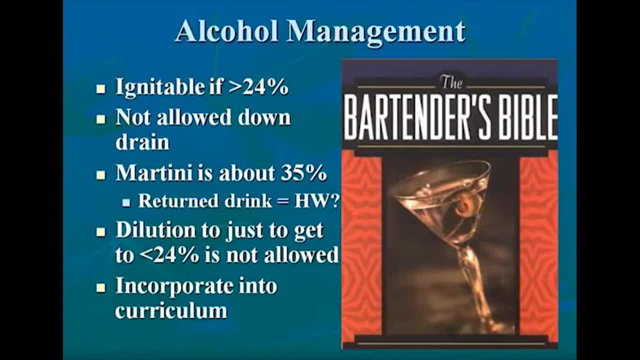 I'll find a 55-gallon drum of flammable liquids. I'll very carefully pour it in there and close it. I'll write the accumulation start date and start disposing this as hazardous waste. Does the bartender do this? Absolutely not. As a hazardous waste inspector do I get to inspect bars? 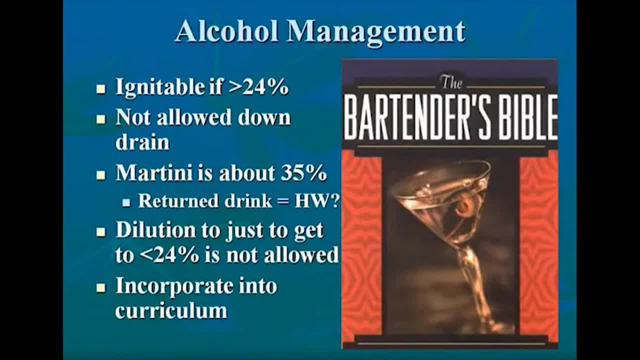 Absolutely not. It kind of looks bad when the county vehicle is driving up to the front of the local tavern and I disappear for an hour to do my job, My very in-depth inspection, in there. So are you going to get busted by a hazardous waste disposal inspector if they catch you? 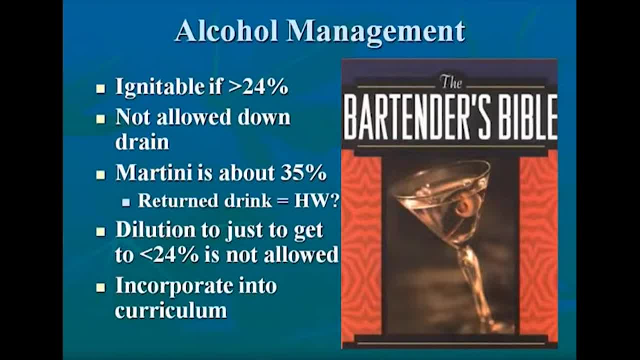 pouring a little bit of alcohol down the drain? Probably not. However, as a well-trained hazardous waste inspector, am I going to recommend that you pour your alcohol down the drain illegally? Absolutely not. You should collect it like large generators of alcohol do. 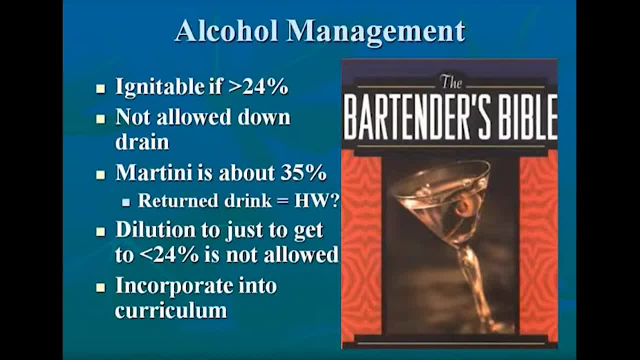 Collect it as flammable, hazardous waste, ship it off for disposal. One thing you can't do- That's pretty sneaky, though- is there's a great laboratory exercise you can do with alcohol. If you take 100 milliliters of alcohol and 100 milliliters of water and you combine them. 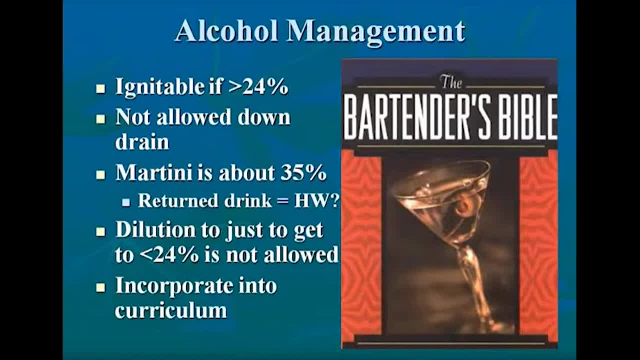 they don't add up to 200 milliliters, They probably add up to maybe 180 milliliters. Now how does that work? Well, it actually involves the molecular structure of these two compounds And if you happen to have, the dilution in that process be such that you end up with 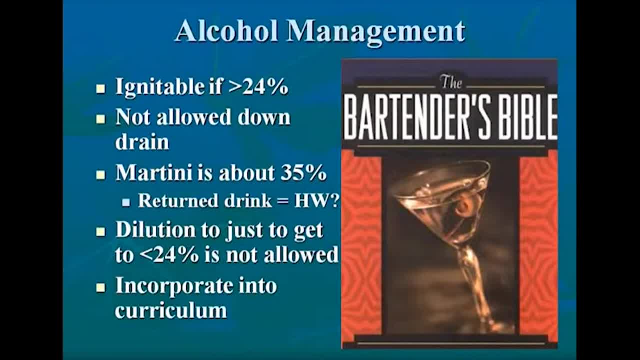 less than 24% alcohol. Again, it's not waste disposal, it's not dilution. What you're doing is showing this chemical property At that point when you're done using it as a teaching tool. now it's a waste. 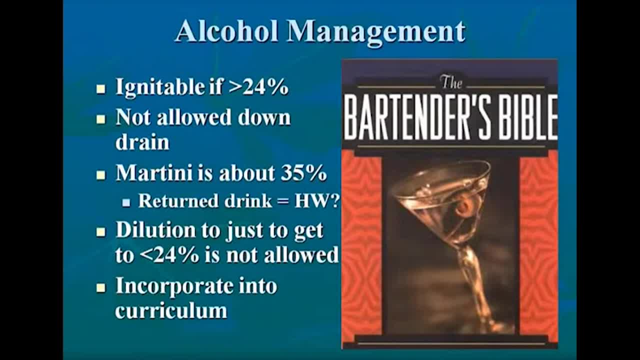 For something to be hazardous waste, it has to be a waste, and then it has to be hazardous. If, at the point where you say, all right, this is now a waste, I can't use it in my curriculum anymore. If it's less than 24% alcohol, it's not hazardous. 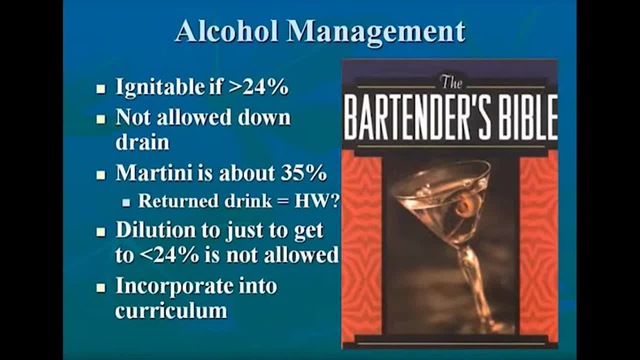 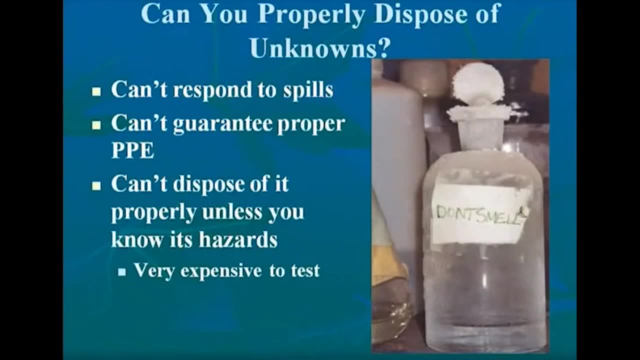 If it's not a waste- hazardous waste- you can pour it down the drain because it's completely water soluble. So that's a way, not necessarily around the law, but a way to actually use your waste alcohol as a product. so it's not really a waste. 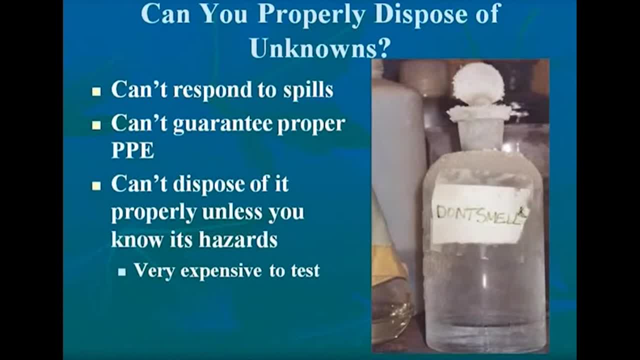 One of the things I want to mention here is that you can't just dispose of hazardous chemicals any which way you want. If it's an acid, it's going to go to a commercial site and be neutralized. If it's flammable, it's going to be going off to be neutralized. 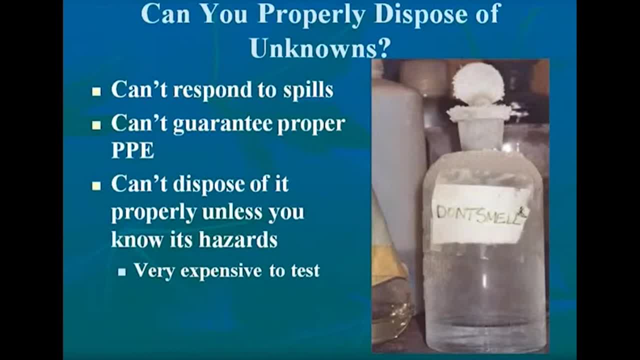 If it's an acid, it's going to go to a commercial site and be neutralized. If it's an acid, it's going to be going off to be incinerated. If you've got an unknown compound like our, don't smell here. you don't know what the 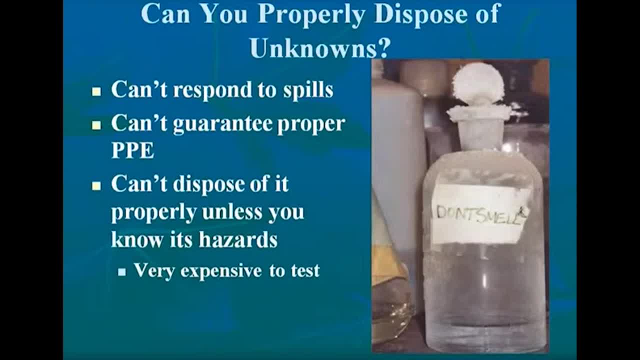 hazardous characteristic is: If you don't know that, you cannot get it taken away from you for disposal, And if it spills you don't know how to respond to it. So unless you know it's hazardous, you can't dispose of it. 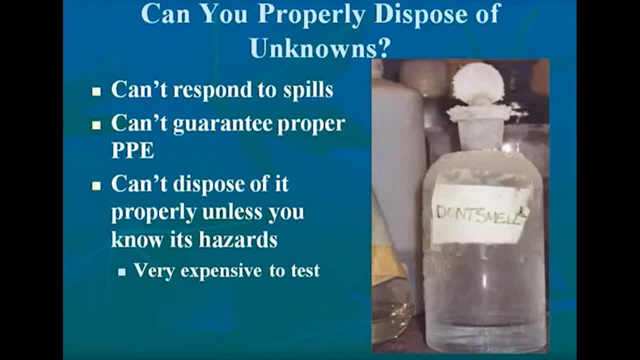 And if you don't know the hazard, you're probably going to pay somebody else to figure out what those hazards are. Those types of tests can be very expensive. These ones can be found in old labs like this one that's down in a basement. 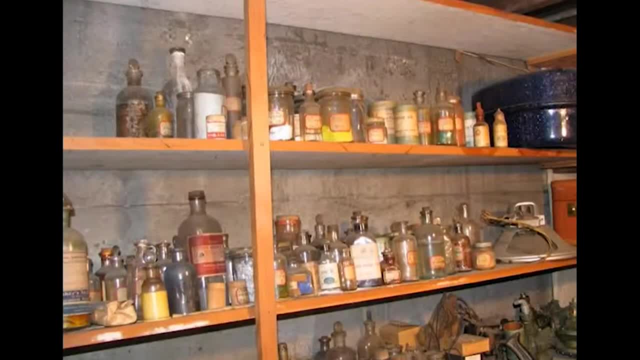 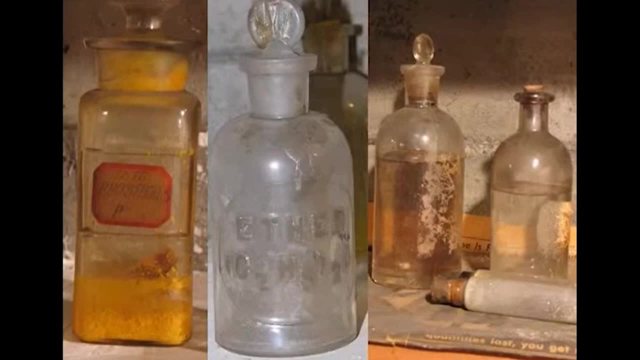 And they could turn out to be extremely explosive. They could turn out to be water. A clear liquid like this, ethyl ether, is a potentially explosive compound. It looks exactly like water. So the clear liquids and the white powders in a laboratory setting are ones that pose. 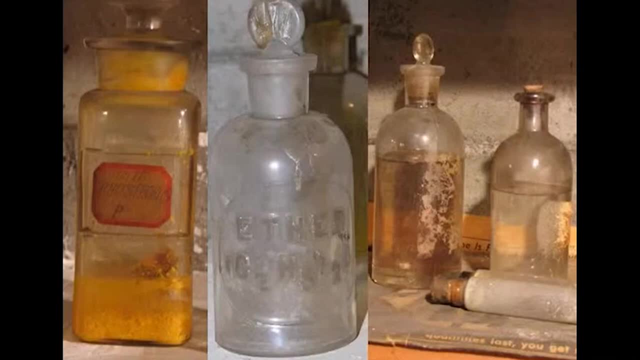 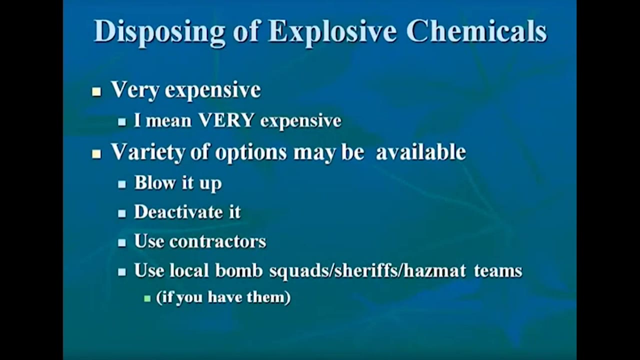 particular risks if they're not labeled. So label your chemicals so you can ensure that they're properly disposed. If you do find explosive chemicals and have to pay for disposal, it's not going to be very expensive, And I mean very expensive- thousands of dollars per bottle potentially. 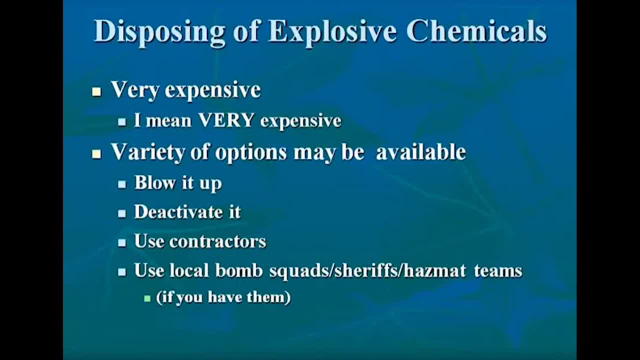 There's a variety of options that may be available depending on where you're located. Some places they blow it up. They'll take the material out, shoot it with a gun- Not you, a professional. Shoot it with a gun and have it detonate. 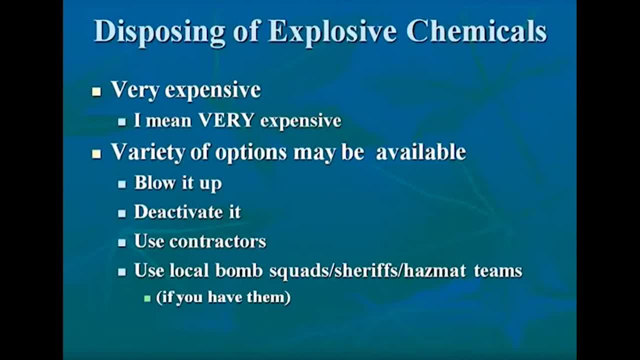 You're not allowed to do that. Shooting hazardous chemicals is kind of forbidden under most laws. But if you've got a sheriff's department or a bomb squad, that may be an option. That may be what they do. They may wrap it up with detonation cord offsite. 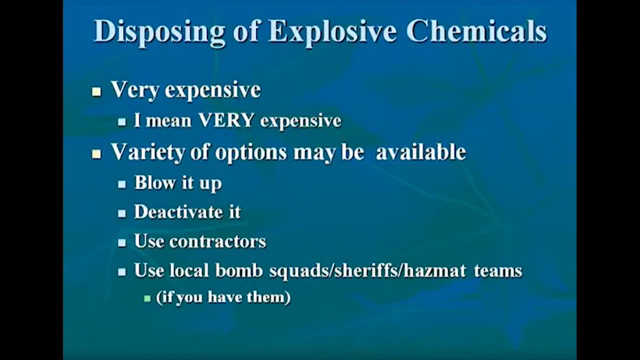 The challenge, of course, is trying to get it out of your school out to a place where they can do that. Shooting it inside the school is really not recommended. There are chemical deactivation contractors, which is what we've been using in King County. 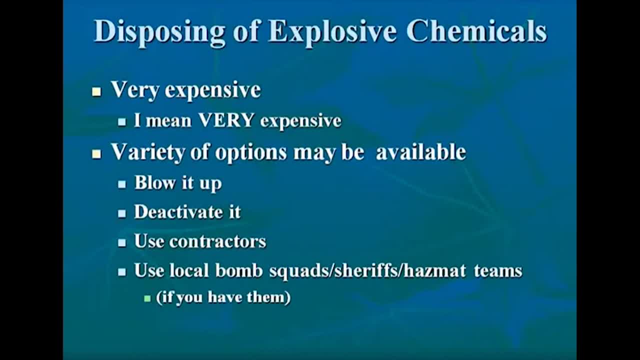 They're under a state contract And you can contact me. I'll be providing my contact information in just a second about how to get ahold of these people. if you should find bombs at your site, Check around before you start looking for these things to see if your local sheriff's